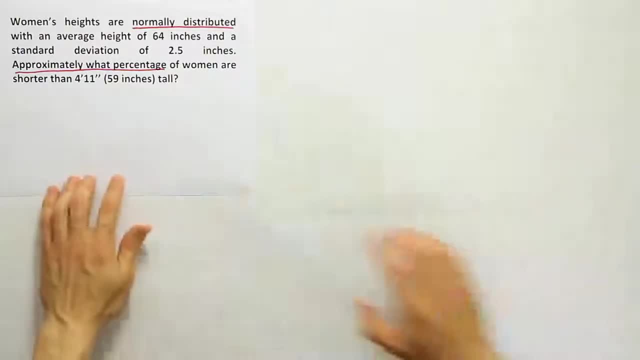 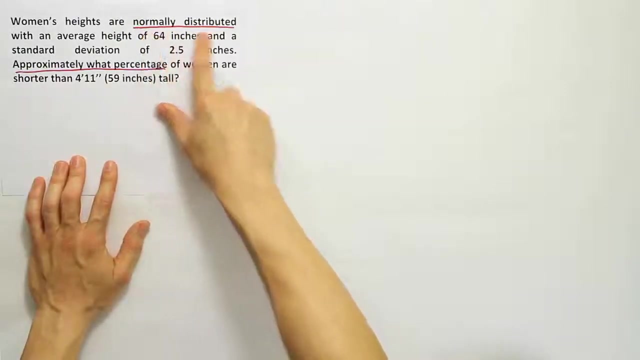 Okay, women's heights are normally distributed, with an average height of 64 inches and a standard deviation of 2.5 inches. Approximately what percentage of women are shorter than 4'11 or 59 inches tall? So I've underlined some key phrases here. Normally distributed. 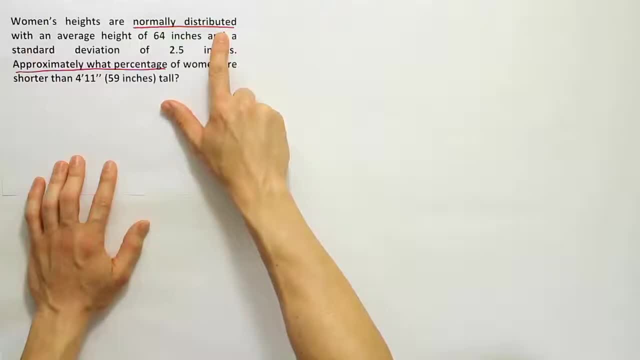 jumps out at me in this problem. That's indicating that we're dealing with a bell curve, So women's heights fall under the bell curve shape distribution. They tell us the average to standard deviation and they ask us approximately what percentage of women are shorter than this in the height. 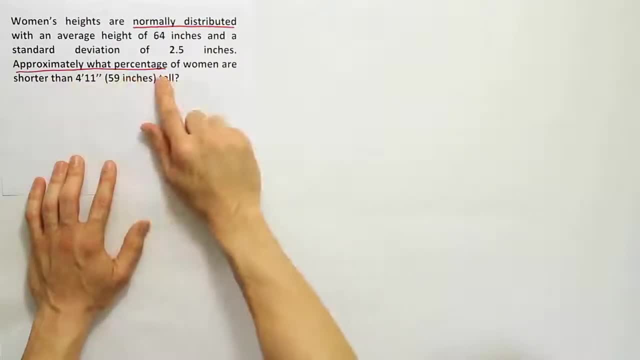 here This approximately what percentage is another key phrase to indicate empirical rule. So the fact that we're dealing with something that's bell shaped and they ask: approximately what percentage, as opposed to the minimum percentage, or at least what percentage. Those phrases, when it says minimum, or at least correspond to Chebyshev's theorem. Approximately, is the 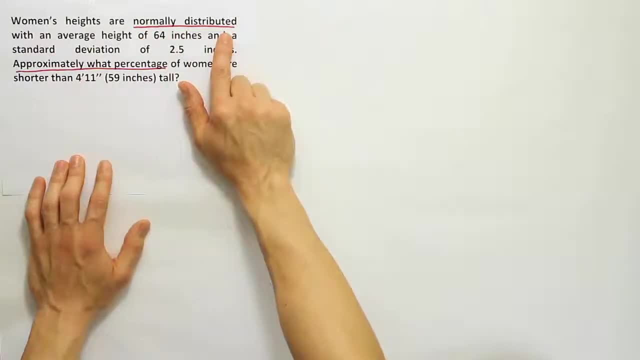 language we use when we're dealing with the empirical rule and normally distributed is required for that rule. You must be using a bell curve to use the empirical rule And if you combine that with this phrase here to me, it tells me that this is an empirical. 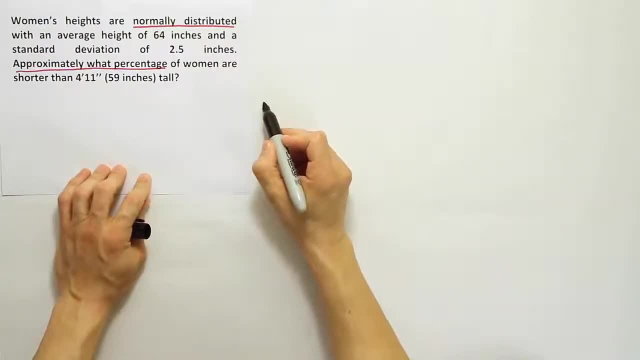 rule problem. Whenever you're dealing with an empirical rule problem, I recommend drawing the bell curve. I think that's very helpful. So we're going to go ahead and draw a bell shaped curve as best as we can here, And I'm going to label the information from the problem. 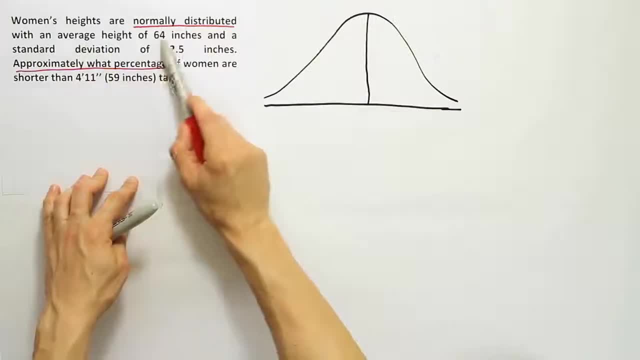 on the curve. So what I'm going to do is look at this average height of 64. I'm going to go ahead and label that in the middle And I'm going to call that the mean, And then I'm going to go on to say that. 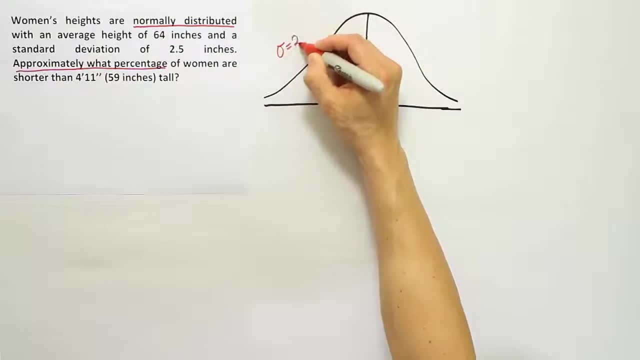 The standard deviation is two and a half And I'll put that up there in the left hand corner. Okay, from there. what I want to do normally is I want to figure out what side of the curve the number they're talking about is on. In this case, I think 59 is clearly. 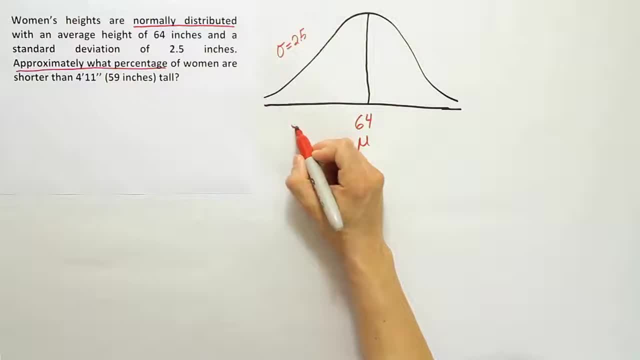 less than 64. So I'm going to go ahead and put 59 somewhere here on the curve to the left of 64. And I'm going to draw a line indicating where that would be on the curve above. Now they want to know the percentage of women that are on the left of 64. And I'm going 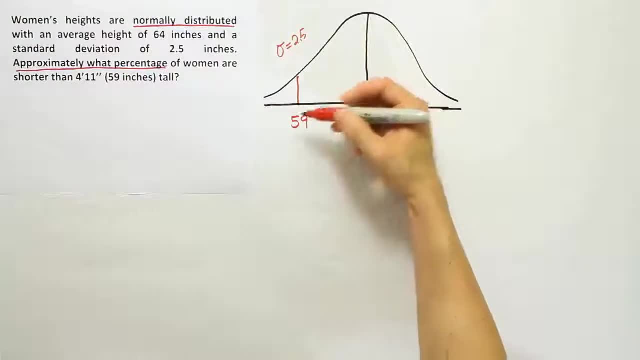 to draw a line indicating where that would be on the curve above. Now they want to know the percentage of women that are shorter than this height. So shorter means to the left. These are the people who are shorter. These people are the ones who are 58 inches. 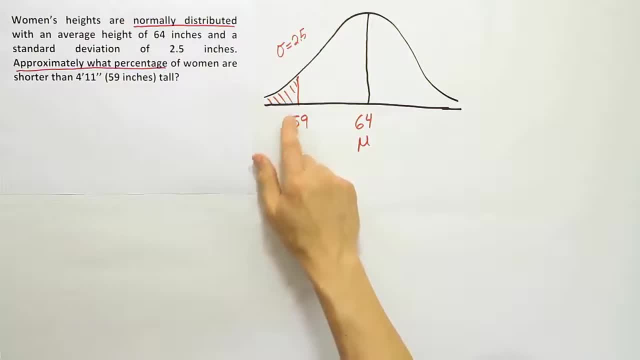 57, so on and so forth, And I want to know approximately what percentage is contained within that area. Alright well, if I draw a little mark here indicating the halfway point between these two numbers, And I'm doing that because what I want to do next is I want 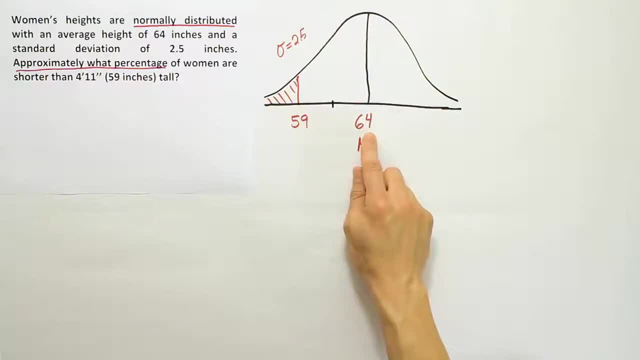 to figure out exactly how far away is 59 from 64. There's a couple ways you can do that. You can actually do it in an equation, And in that case it's kind of like finding k in Chebyshev's theorem. So you can say: let's take the value 59 and then subtract off the. 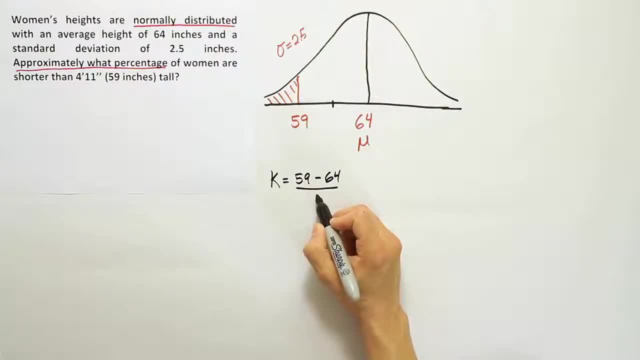 mean and divide by the standard deviation, which is two and a half, And when we do that we end up with 59 minus 64, we end up with a negative five right And then we divide by 2.5. And we see two and a half goes in that twice because it's two standard deviations. 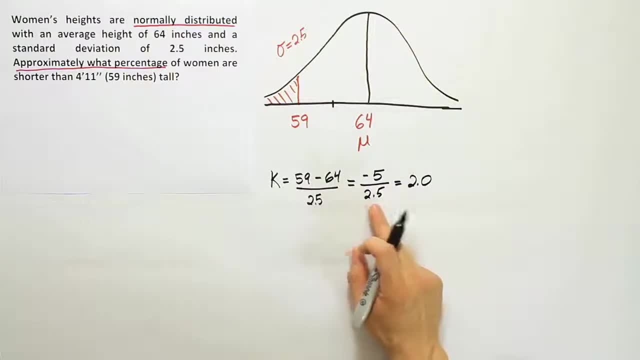 It's two standard deviations away from the mean, If I count by two and a half, which is another way to do it. By the way, this is negative. The negative just indicates that you're below average, right, So don't really worry about that as much. We're more concerned. 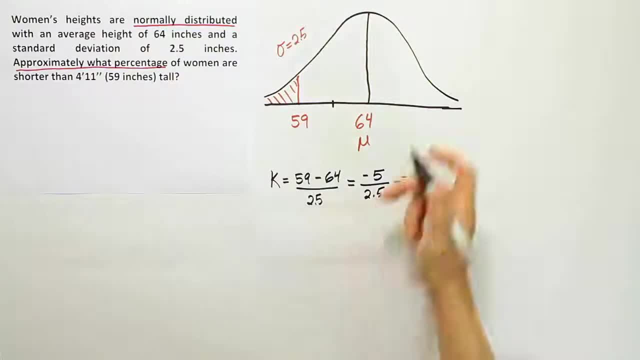 with the absolute value of this number. Now back to the idea of counting by two and a half instead. we could also do that. We could say: well, if I go from 64 and I take away a two and a half, I'll end up with 61.5, right, 61.5.. That's kind of the number here, And 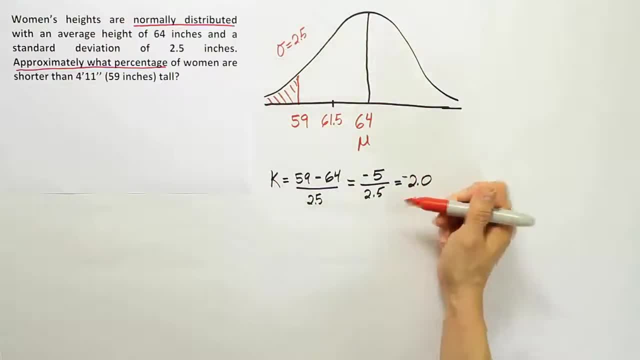 by two and a half, I end up at 59. That's another way to figure out that it's two standard deviations below average. One, two standard deviations below average. Okay, And once I've figured out that, then from there I have to work with my rule. So I have to know Chebyshev's. 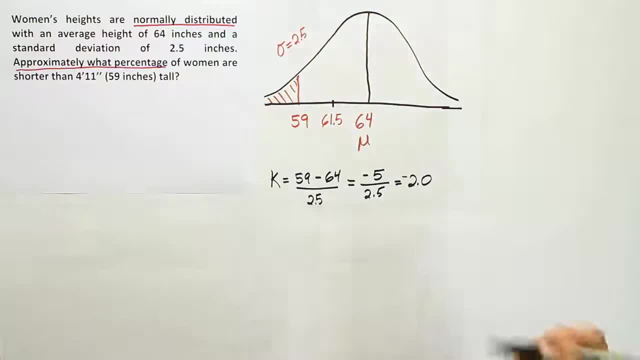 rule, or sorry, the empirical rule, and figure out what it tells me. So we have some rules. We say that when k is equal to one, that corresponds to 68% of the data approximately. When k is equal to two, it corresponds to an interval that captures 95% of the data. And when k 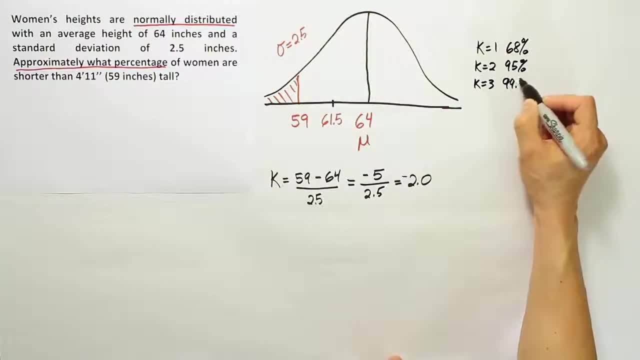 is equal to three. it corresponds to an interval that captures 99.7% of the data. But we want to do kind of a little drawing here to help us see. when they say 68%, what are they talking about? Well, 68% is dealing with one standard deviation away from the mean. So that's just. 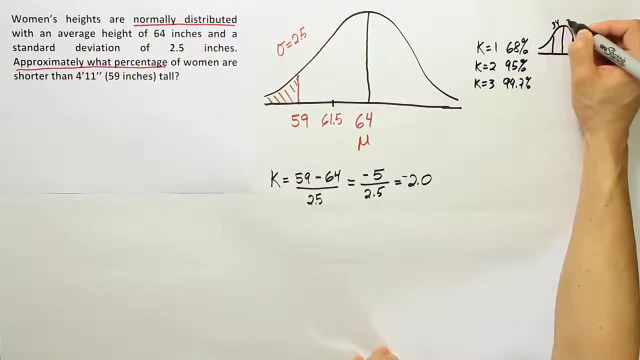 one standard deviation away, And that'd be 34 and 34 on each side For the two standard deviations. we're talking about a scenario where you're working from four and a half, not one, but two standard deviations away, And so in that case you have half of 95 on each side, or 47.50 in each piece. 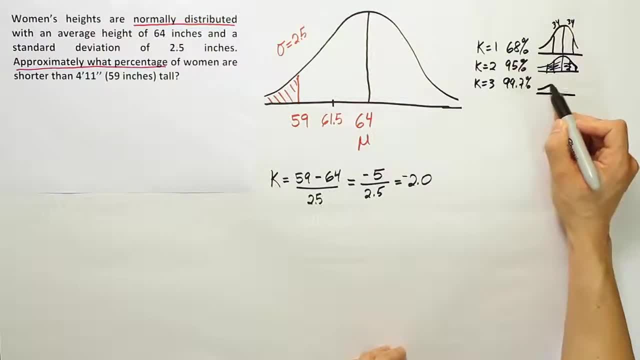 Alright, then, finally, the last one obviously would be three standard deviations, And again, trying to squeeze in these little drawings is difficult, but it would be three standard deviations, half of 99.7 on each side. Okay, so, regardless of that information, what we're going to do then is to think about. 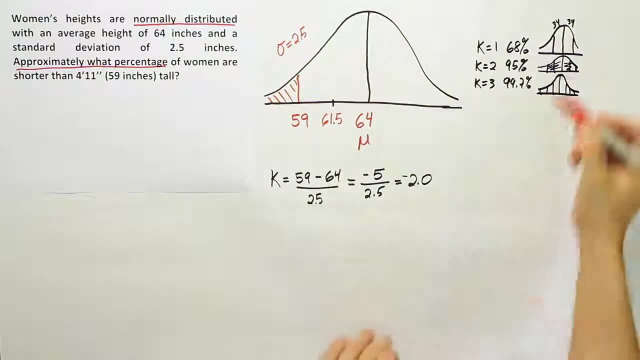 how we're going to determine this, because we have drawings that talk about what's in between right, What's in between one standard deviation above and one standard deviation below. This one is two above and two below and this one is three above and three below. 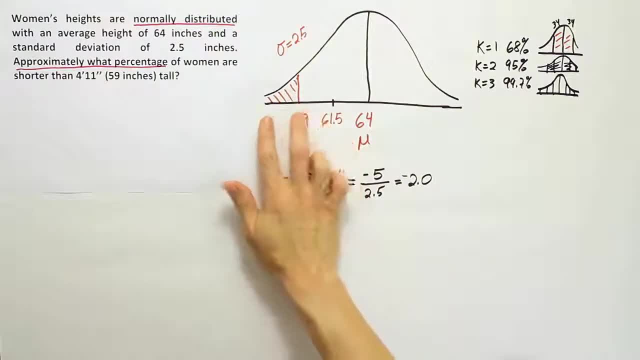 But our question is, though: how do we work a problem like this where we're talking about just a little sliver outside of two standard deviations? Well, it means, you know, since our k was two, we should be looking at this kind of a drawing and trying to think about it. 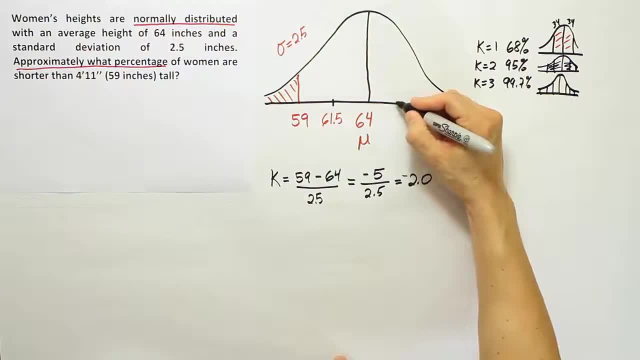 So I'm going to draw a standard deviation marker here and one here and I'm going to say: hey, look, from this span to this span, this whole distance here that's 95%, right, But each half, because the curve is symmetric- each half is 95% divided by two. 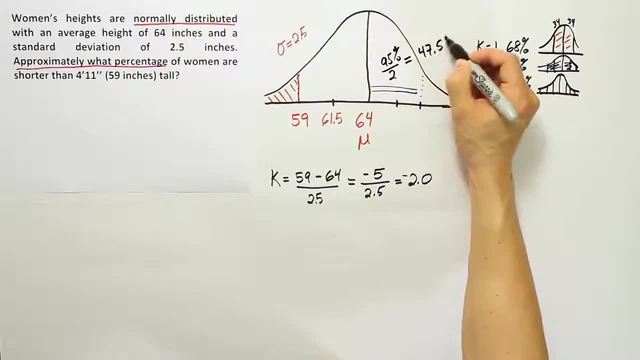 And that's going to work out to be 47.5%. if you either do that in your head or in your calculator, That means that this half is also 47.5%, for the same reason that the other half is right. 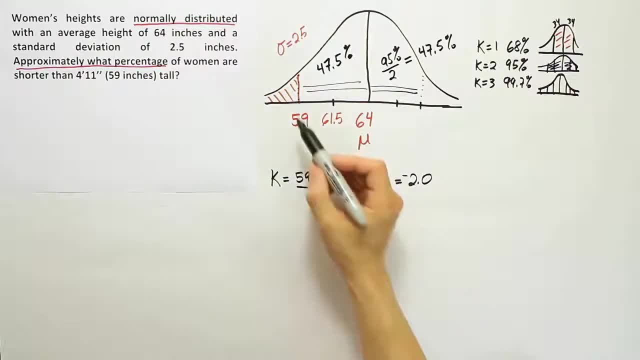 It's symmetric, The two sides of the curve are equal, Then what we can figure out is: okay. well, if this total span is 95%, this tail and this tail have to add up to the remaining 5% to give you 100%. 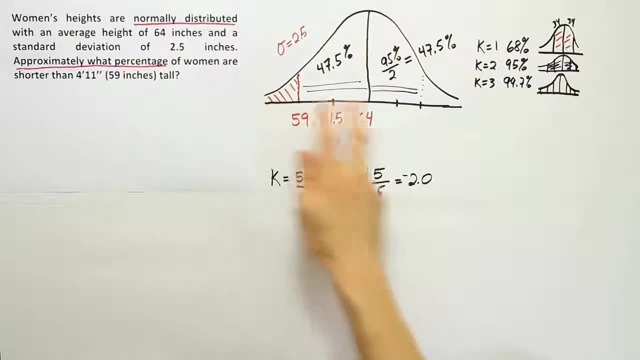 So if it's symmetric, this must be 2.5%, this must be 2.5%. That's one way to think about it. The final way to think about it, and the way I think is probably most useful, is to realize that, look this, half of the curve, from here over, all the way over, must contain 50%. 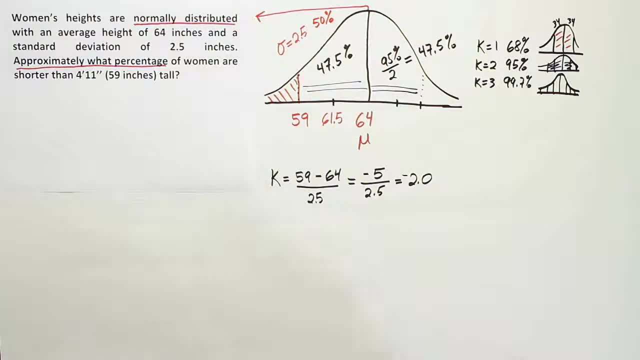 That must be true, because it's half of the curve. From the mean over it's half of the curve. So if that contains 50% of the data and this amount is 47.5, then what must this be? Well, you can just subtract them, because we know that this space plus this space adds up to 50.. 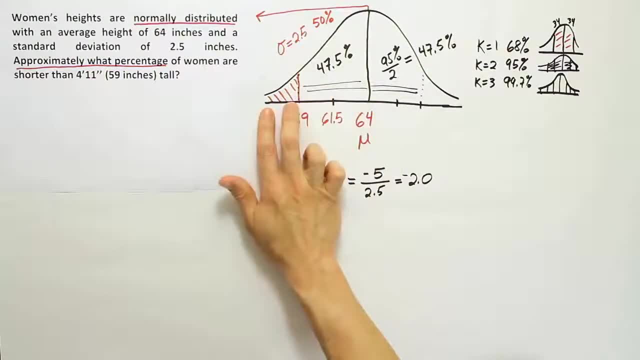 So if I take 50 and take away the 47.5, I will get 2.5%. So that's going to be my final solution. the approximate area That is less than 59 inches is equal to 50% minus 47.5%. 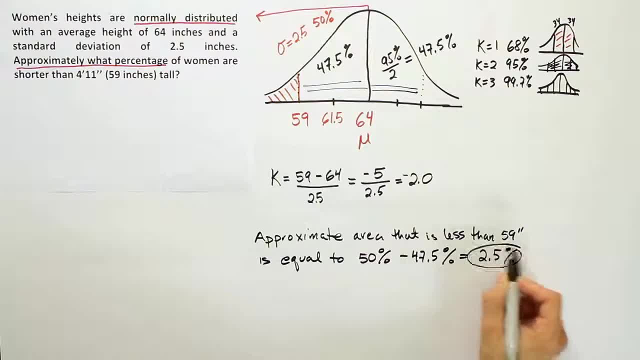 And of course that's going to be 2.5%. Again, it's a good idea to do the drawing so you see this clearly. but if we add 47.5 and 2.5, we will come up with a full 50.. 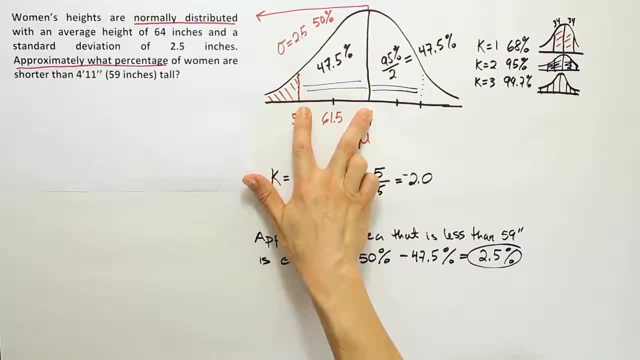 And just to recap, the other possible way to think of it is to say: look from here to here, the two spans, the two positions when k is 2, two standard deviations below two standard deviations above the mean that span captures 95%. 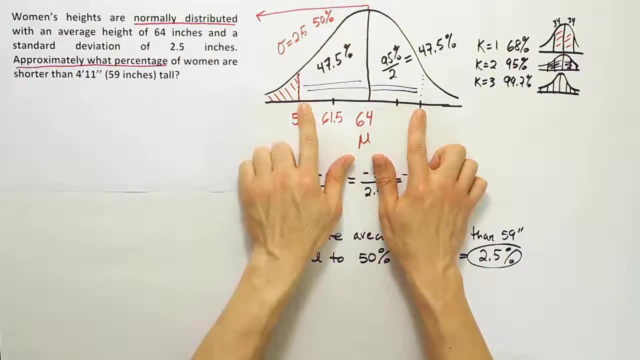 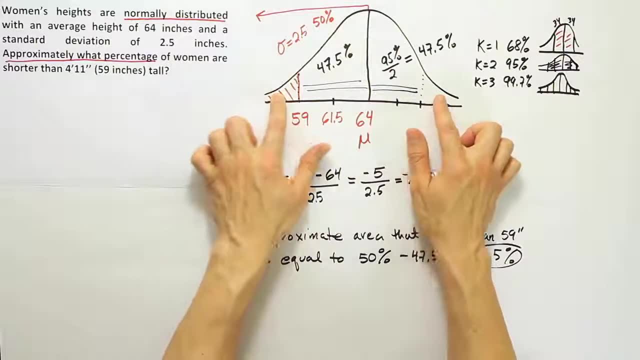 So from here to here is 95%, It must mean that outside of that this area must be just 5%. And if it's 5% and the curve is symmetric, each one of these tails here, they have to be 2.5%. 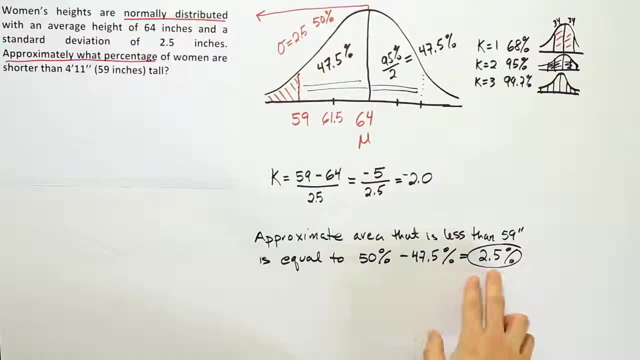 That's another way to reason. Wherever you reason it, though, the answer turns out to be 2.5%.